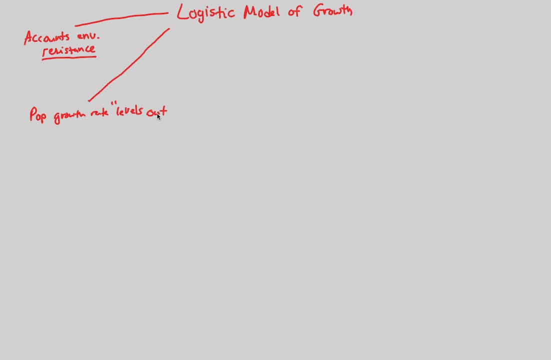 Population growth rate levels out- that's the term we want to use here, meaning that at a certain point there's going to be a leveling And that, specifically, is going to be to zero, When the environment's ability, when ENV's ability. so remember the environment. 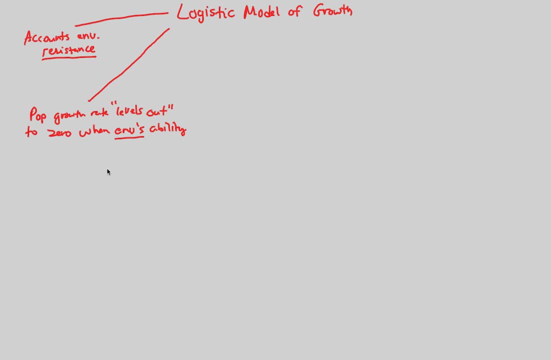 this is the non-living portion that we're talking about. the environment's ability to support population is reached, Meaning that the resources have been met. they've been reached. there are no more resources. all the mates have been taken. they cannot reproduce anymore. all of those things. 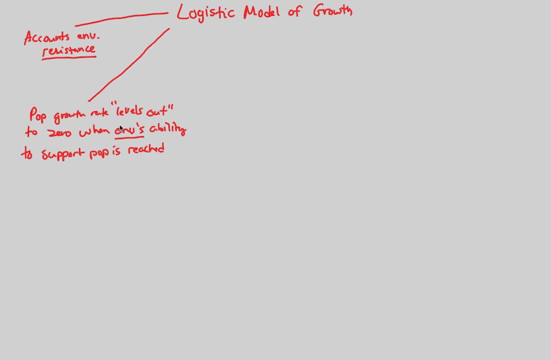 all of those resistance and limits, limit ideas, have been met and thus the population growth rate levels out. This leveling out, this reaching of the environment's ability to support, that is actually called reaching the carrying capacity, And that's what we're going to entitle the next part of our flowchart. 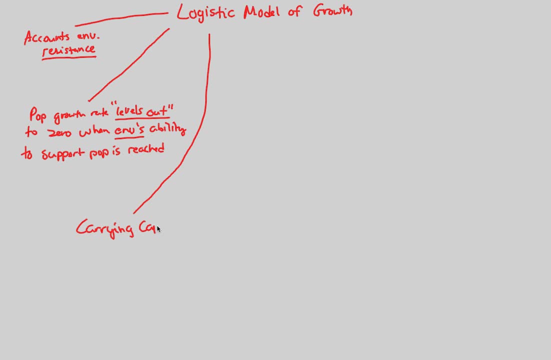 The carrying capacity is the term that we use. when we say that a population has reached a certain level of zero, let's say growth. And that's when it reaches a certain level of zero, let's say growth. And that's when it reaches a certain level of zero, let's say growth. 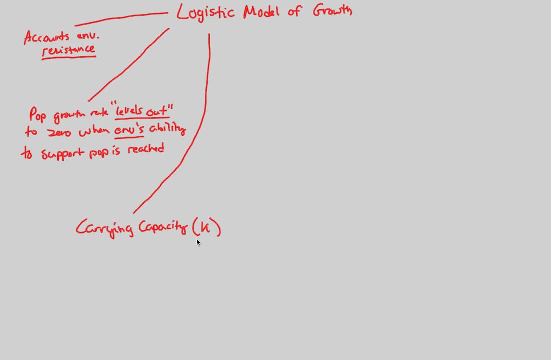 That's when it reaches carrying capacity denoted by the letter capital K. Carrying capacity is going to be further defined, based off of this idea, as the largest population that can be maintained for an indefinite period. for an indefinite period, and specifically by a particular environment, by particular 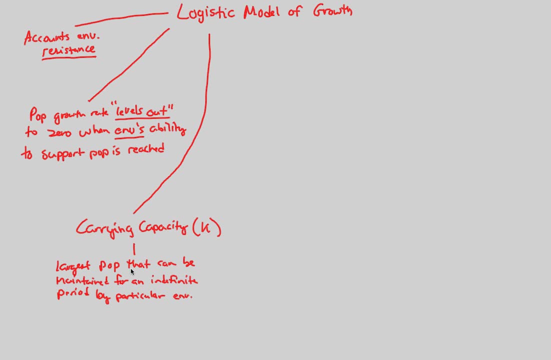 ENV for environment: The largest population that can be maintained for an indefinite period by particular environment. Big idea here- so I want to put a star here- is that there's going to be an assumption and that assumption will be the following: The star here denotes that there. 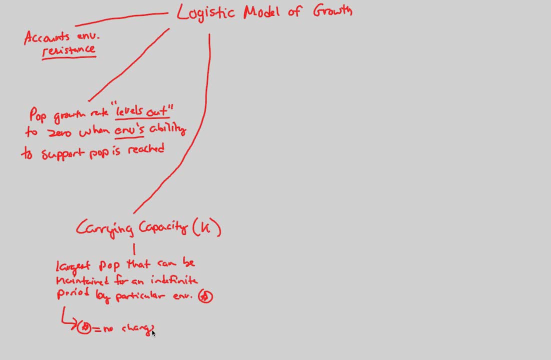 are actually going to be no changes in environment. If the environment stays stable, if there are no changes whatsoever, you're going to reach a carrying capacity and stay at the carrying capacity. The best way to understand carrying capacity, the best way to understand this leveling. 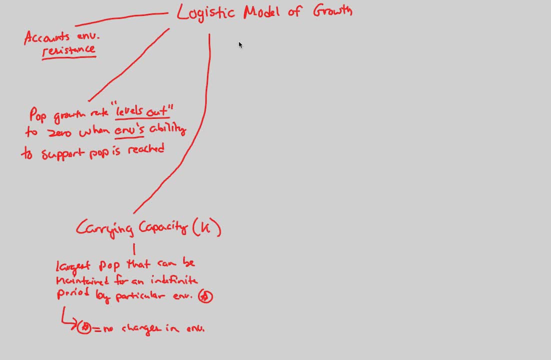 out this resistance that's being met is to look at the actual shape of this graph, And that shape of the graph is called an S-shaped graph. It's S-shaped, that stands for a sigmoid curve, S-shaped curve. That's what our graph is going to look like And specifically, we have to. 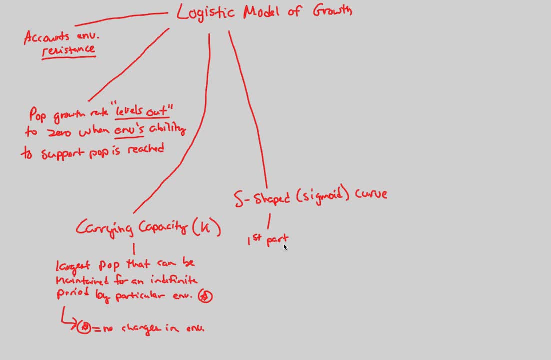 first mention that the first part of the curve- this is of note. it's quite interesting to see that the first part of the curve is indeed exponential. A part of this graph does show exponential. So it would be false to say that no exponential growth is ever seen in populations, because 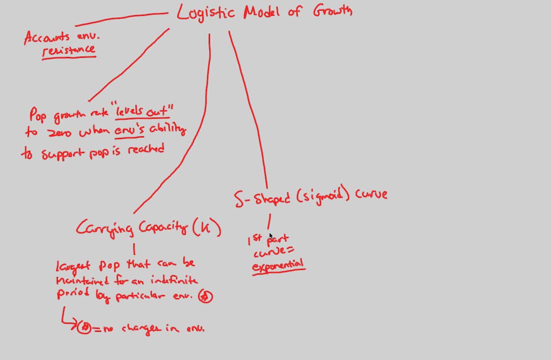 populations are always resisting and fighting things that the environment can't possibly support. That's wrong, because the first part of the curve is indeed exponential, as you'll see. But what you're going to see is that, once K is reached, remember what is K. K is the 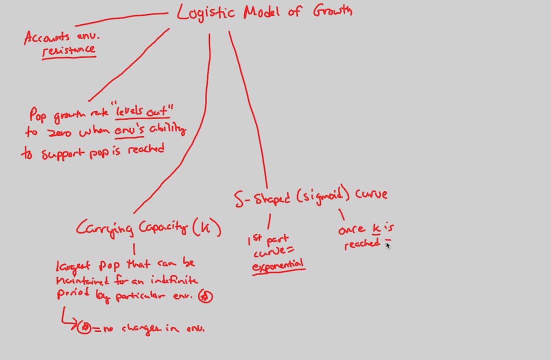 carrying capacity. Once that final resistance has been met, we're going to have a leveling out. The population levels out. You'll see what I mean right now. So let's see. We have a graph. What's on the side? The side, the y-axis is population size, denoted by capital N, And over here we simply have 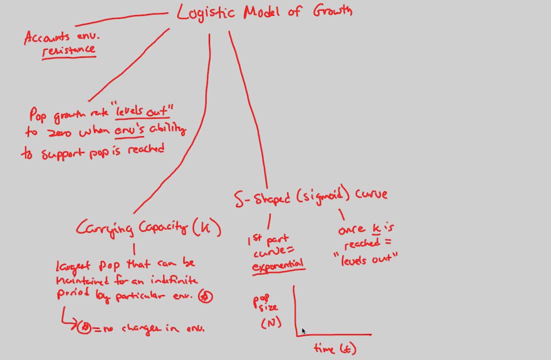 time denoted by lowercase t. This is our sigmoidal curve. It's a very simple idea in mathematics. You've probably seen it before. This is a sigmoid Notice, the S-shape Notice the first part of my curve right over here. Watch my mouse. This right here is the size of the population And this is. 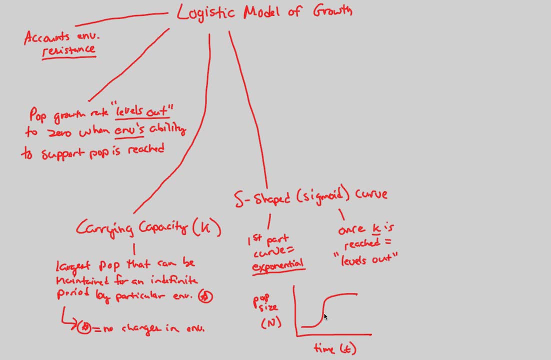 up to this point. That's all exponential growth seen right here. So this is the first initial part, And then I'm going to reach a certain level And that level that I'm reaching I'm going to put it as a dotted line right here. Once I reach this level, 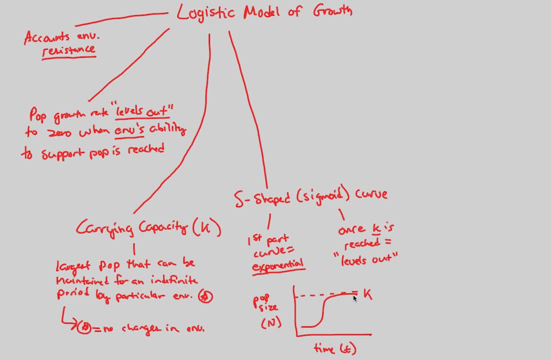 what have I reached? I've reached K. This is my carrying capacity. I have reached the largest population that can be maintained- Look how large this population's size is- for an indefinite period of time by a particular environment. I have leveled out. Look how this was. 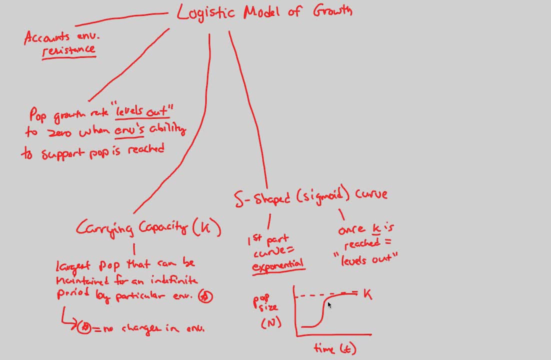 initially growing, didn't it just continue growing all the way up off the screen? Well, that's because you reached k, and when you reach k, you're going to just level it out. and look at, this looks much like an s, thus the name: s-shaped sigmoidal curve, and so 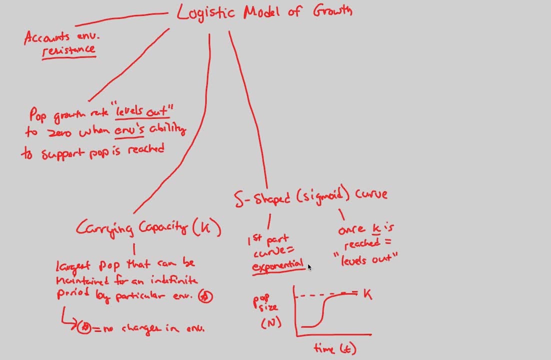 that's a very, very powerful logistical model of growth that we're looking at. Finally, last point to understand, last couple of points to understand, is the following: In this situation, we're going to still look at a calculus driven equation and we're going to say dn over dt is equal to r, instantaneous it's. 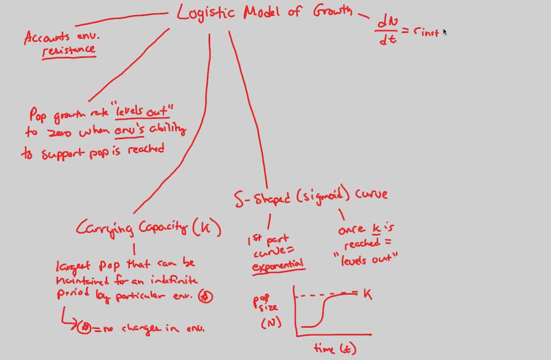 still there. so we're still focusing on that instantaneous rate of per capita growth multiplied by the population size. but now we actually have to involve k, and k is going to be involved in the following manner: it's going to be k minus n. multiply this number, this exponential number, by the fact that there's going to 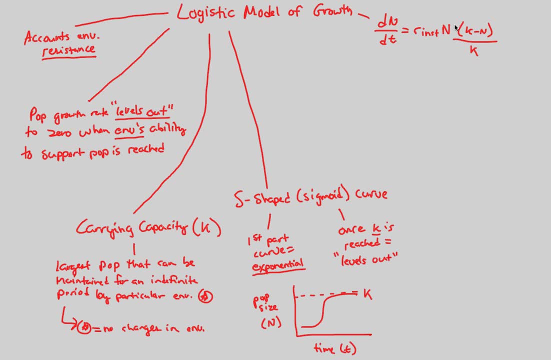 be resistance and I consider this part of the equation right here that we can sort of put in a small little box right here. this addition to the equation of exponential growth- remember, this is outside of the box- is just exponential, but I've added this k scenario and this simply refers to the decline in growth as the 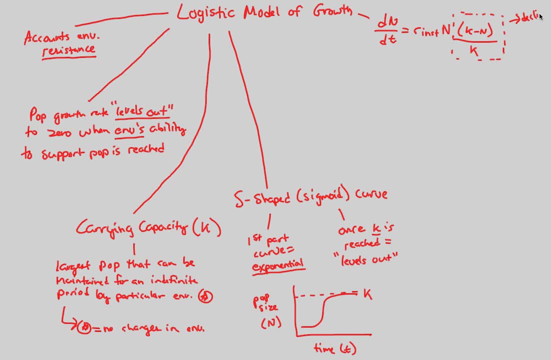 population reaches k, so we're going to write that down. this is equal to decline in growth as population reaches k. sorry for the small writing there: decline in growth as population reaches k. that's what we mean by this boxed in thing, if we multiply this number by the. 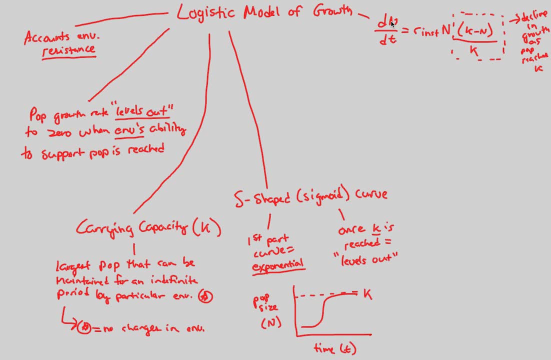 exponential growth, we end up with a sigmoidal derivative, as seen over here. sigmoidal graph- big ideas. to understand. though this is a fancy equation, we just have to understand. the big ideas are the following: if n is small, if our population size is small, it is going to be not. 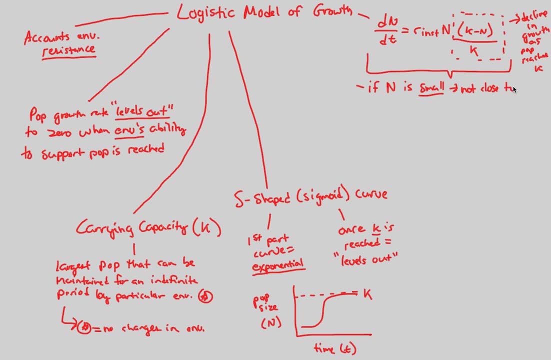 close to k, aka, if it's not close to k, if it's very small and it's not close to k, what we have is the following scenario: We have k minus n, which is that part of the equation over k is about. 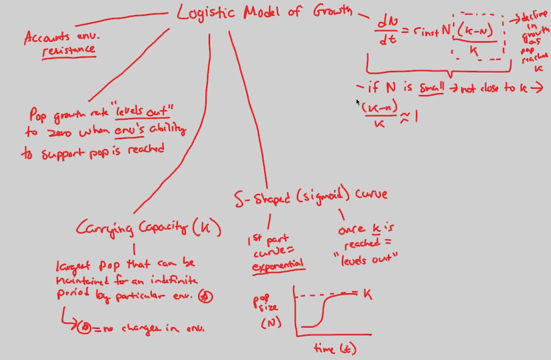 equal to 1.. Okay, this is something you should remember And remember. that only occurs if n is small and if n is not close to k. Both of those things have to happen. you get this final result: What if n is large? If n is large, if there's a huge population, a huge, huge population. 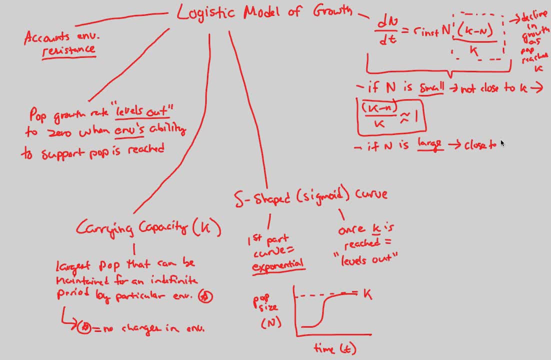 that would mean that n is getting close to k. Think about it. doesn't that make sense? If the population is huge, like, let's say, right over here, aren't you reaching the environment's ability to support the population? Aren't you getting to a point of resistance? Aren't you getting to the 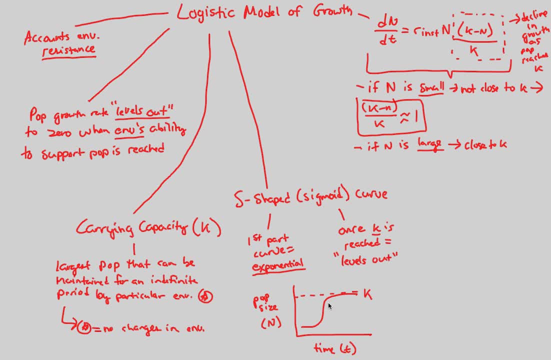 point where resources are about to be limited because there are just too many individuals. And what's the consequence of that? The consequence of that is to level out, And that leveling out, this leveling out right here, means that you're going to have a zero slope. The graph: 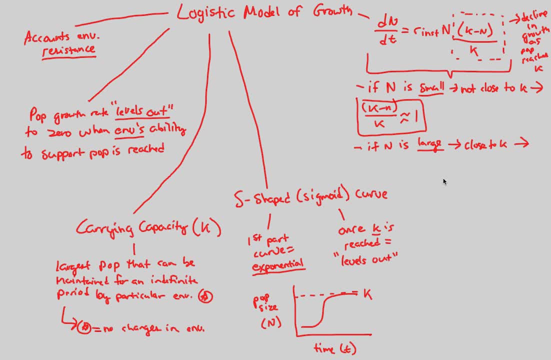 is not going to grow at all, And thus you would expect that this number, this boxed-in idea right over here that we established k minus n over k, is then going to be equal to about zero, Because the population is getting so large. you don't expect that to happen. You don't expect that to. 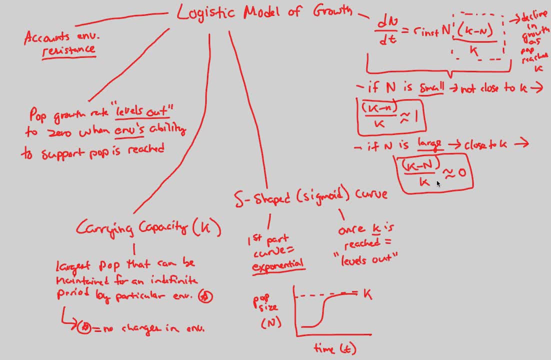 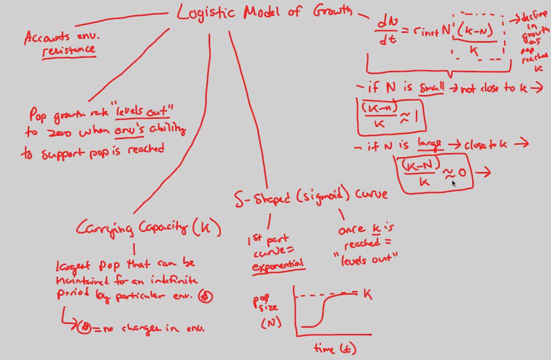 eventually, with this idea of reaching almost zero, you're going to then, of course, going to have a population growth that will decline, And that's just how the math works out on this. That's the big idea here. These two ideas go hand in hand. Over here, the population rate is: 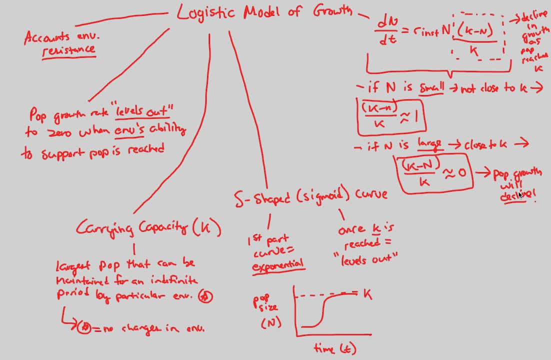 definitely increasing. The number is fixed. The dollar did not, you know, respond. If that happened, You have an increase in population growth. Over here, you have a decrease in population growth. And finally, last point over here, if let's say n is equal to k, 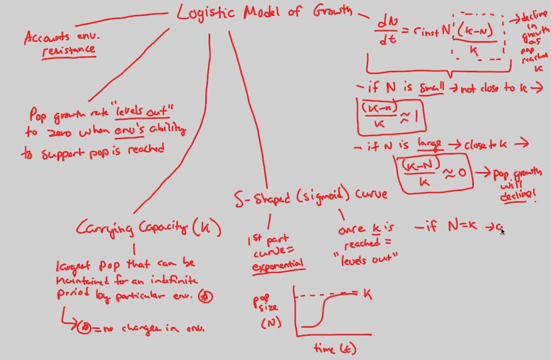 what if you reach that carrying capacity? Then you would state that the growth is equal to 0. That's when it actually is equal to 0. So that's our final point over here, And then, finally, the last thing to understand is always go back to our idea of nature.